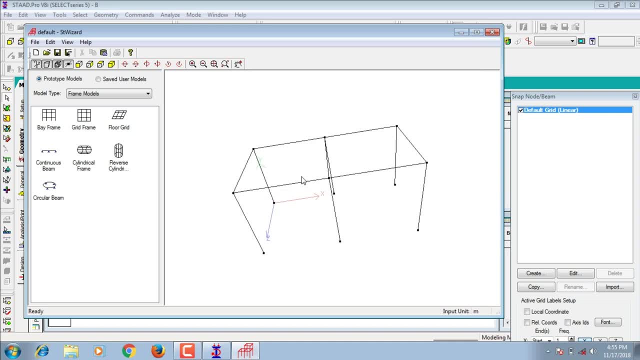 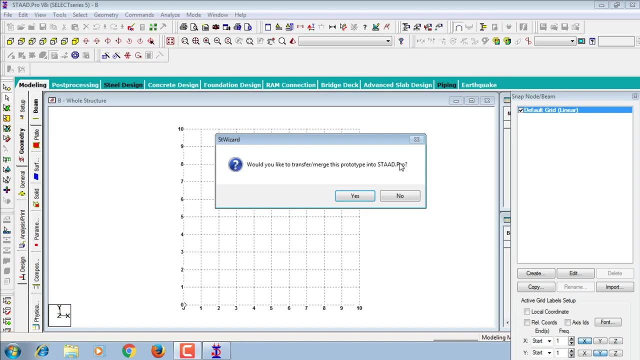 Just apply here. Click on apply. Your frame will be open like this: So this is my frame. I will import this frame to start pro software. Just cancel this. Click on yes button. Click on ok button. So your frame was imported to start pro software. 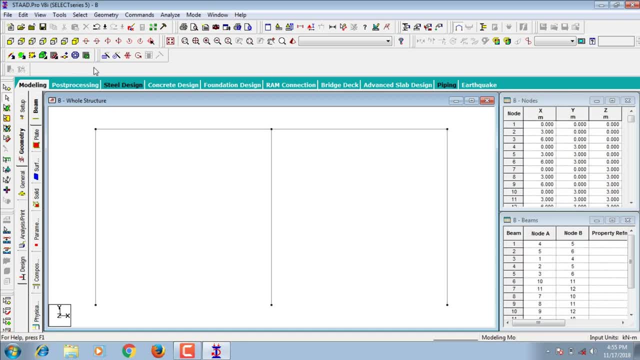 After that, click on hide start node beam button. It will hide your snap nodes, So after that keep your structure in 3D view. For this frame, I need to add slab. For this frame, I need to add the slab. 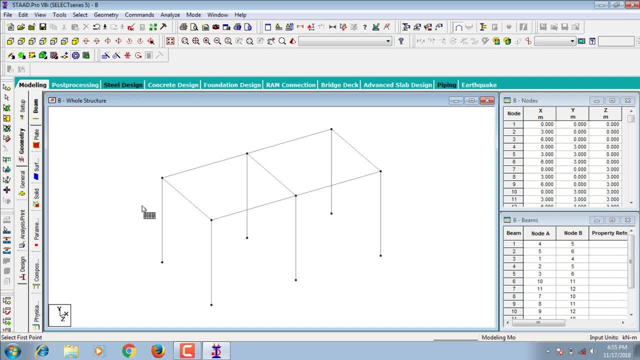 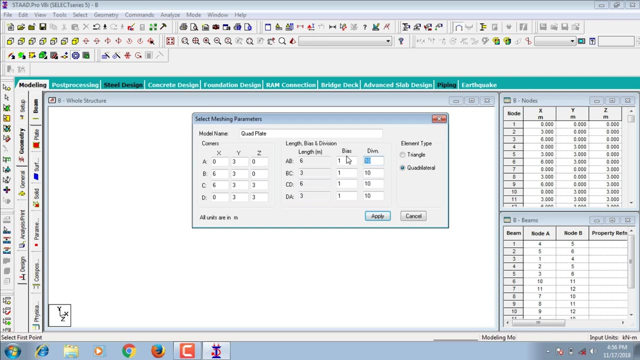 For that go to generate surface meshing. So generate surface by clicking on first point, second point, third point, fourth point, Again first point on the frame, Select quadratal meshing, Click ok button. Just I am assuming number of divisions in A direction, B direction, C direction, D direction. 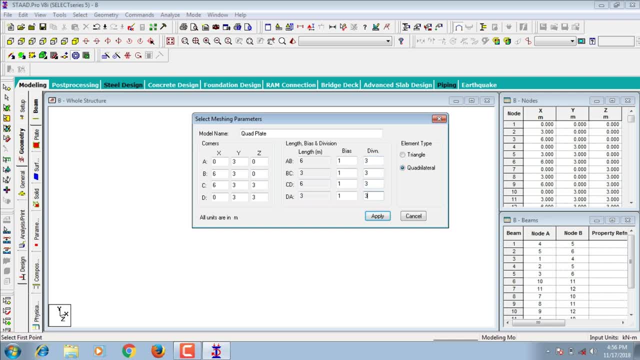 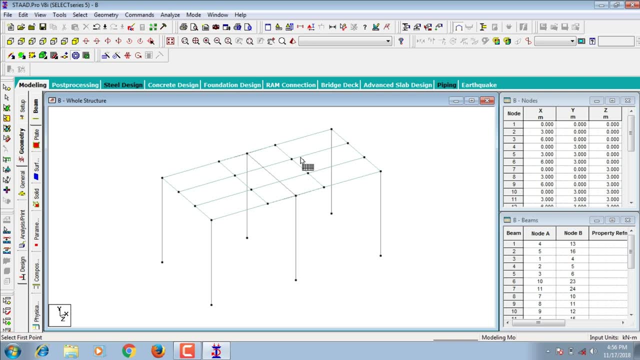 So just, I am assuming 3 on each and every section, Just I am assuming 3,, 3,, 3 along width direction as well as length direction. Just apply here. So it will create 3 number of grids in X direction as well as 3 number of grids in Y direction. 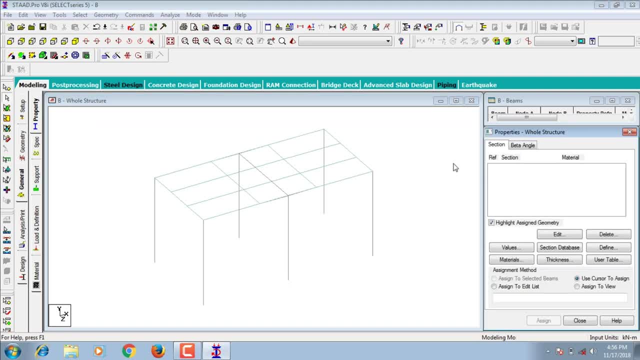 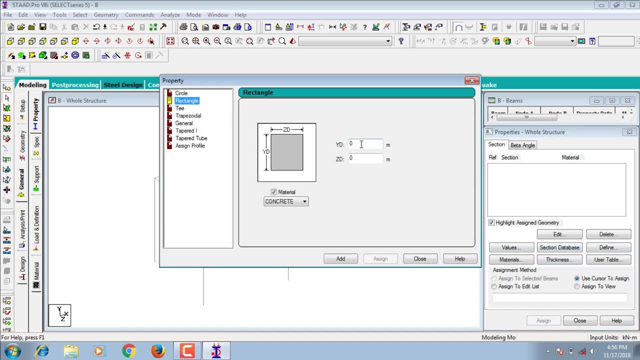 After that go to general. So just, I am giving the dimensions of the beam as well as column for this Go to define Select rectangular. So let us assume beam size of 0.23.. Just add it Again. column size of 0.30. 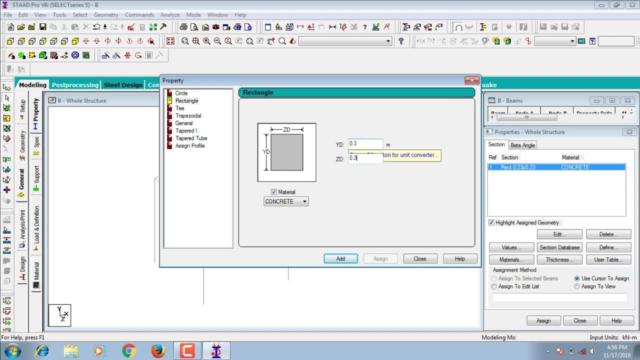 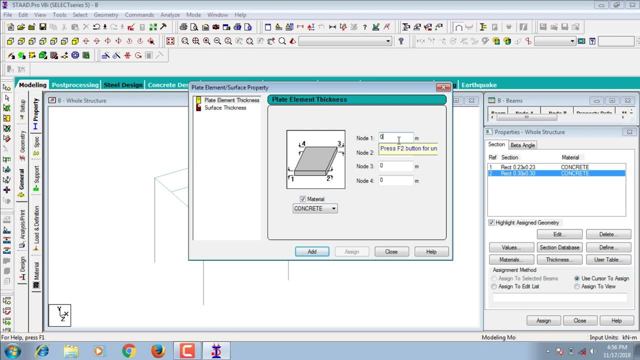 Let us assume column size of 0.30.. Just add it. So after this, go to click on thickness. Just, I am assuming the plate thickness of 0.12.. Slab thickness of 120 mm: Just add it. 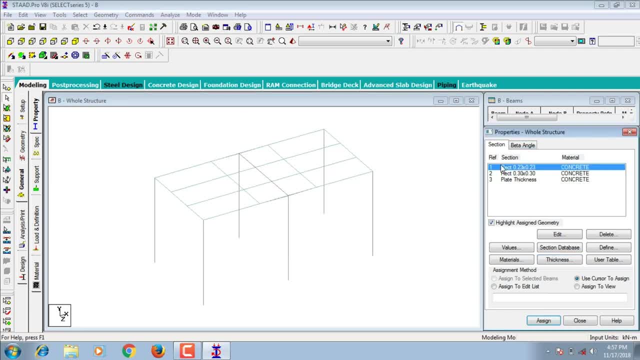 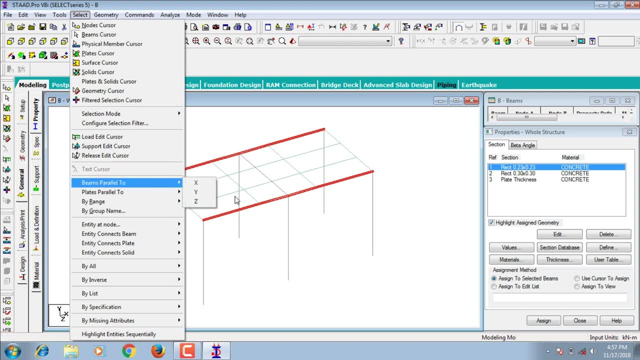 So after that close it Select beam. For assigning beams: just go to select button. Select beams parallel to X direction. Again select beams parallel to Z direction. So click on select to assign to selected beams. Assign Yes. 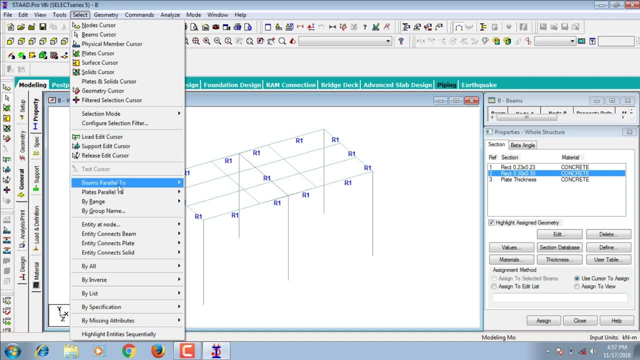 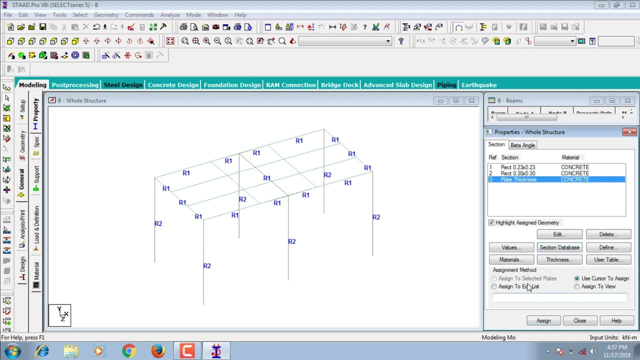 After that, select columns, Go to select again Beams parallel to Y direction. again Assign to selected beams. again Click on next button. Select plate thickness. again Assign to view. again Assign. Yes, I will show this model in rendering view. 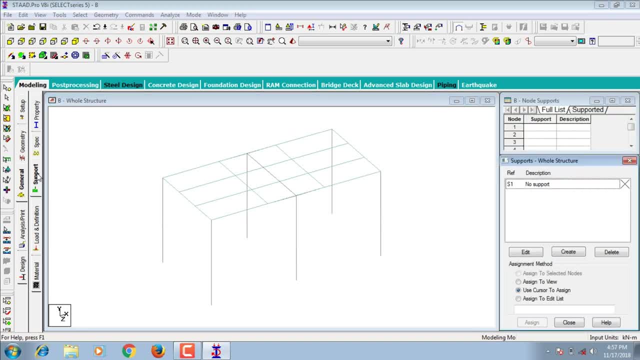 This is my 3D rendering view. So after this, go to supports, So create supports. Just, I am adding fixed support for my frame. Select support 2.. Again, keep your structure in front, view, Select your base node points. 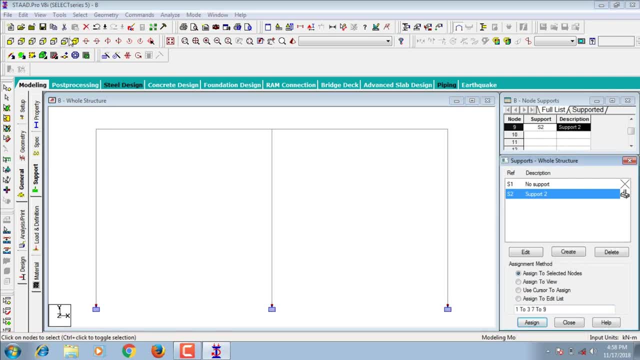 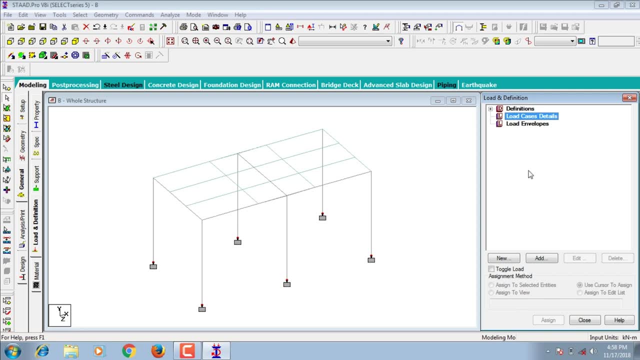 Click on assign to selected nodes. Assign: Yes, So this is my node points. So after that go to loads and definition. Just click on load case details, Just add it. I am creating dead load as well as live load for this building. 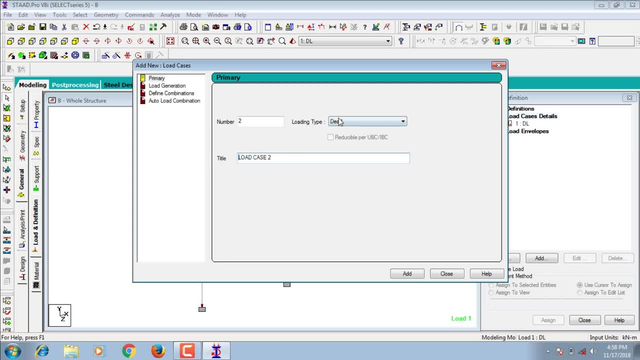 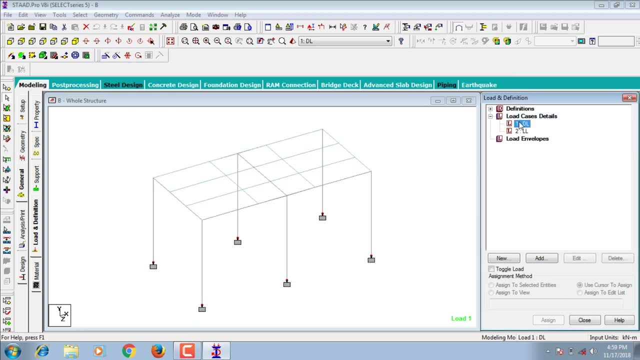 So I was added dead load. Click on live load. Select live load LL. Just add it. Ok, Close it. Select dead load: Just add it. Add your self weight. After that, select live load, Just add it again. 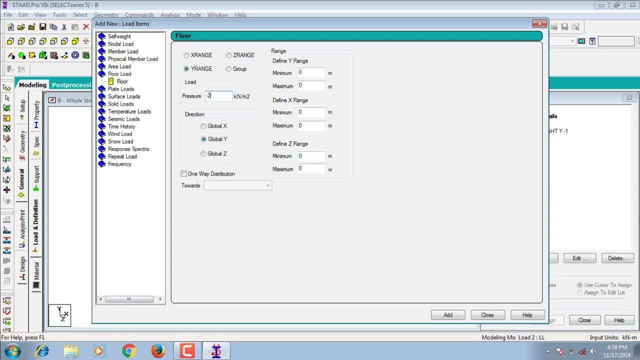 So select here live load as load load. Let us assume minus 2.5 is the intensity. Let us assume minus 2.5 is the intensity. Throw Y direction. My first story was at 3 meter as well as final story was at 3 meter. 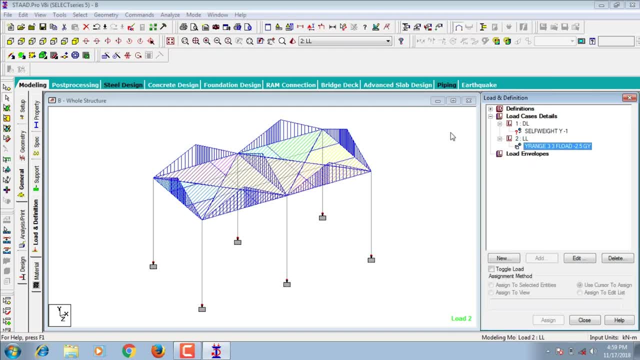 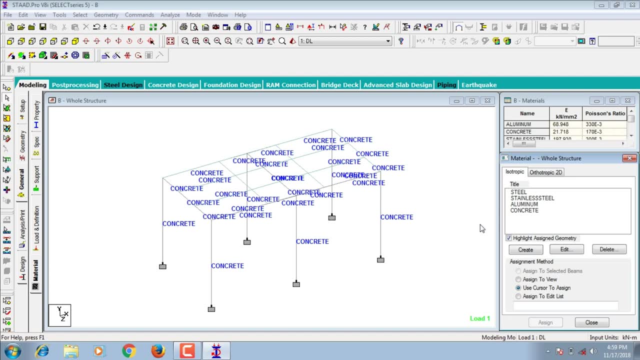 So just add it, Close it. So this is my live load. Ok, After that, select self weight Assign to view Assign. Yes, Ok. So after that go to materials. Ok, Select concrete Assign to view again. 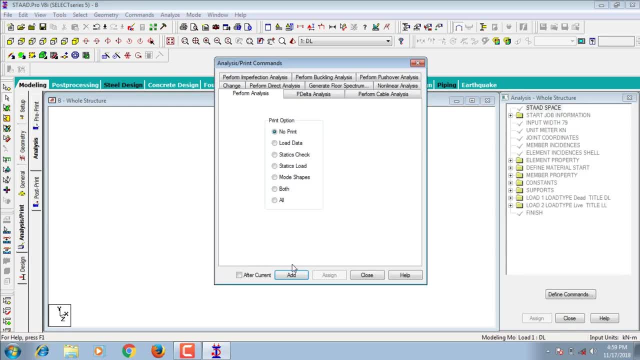 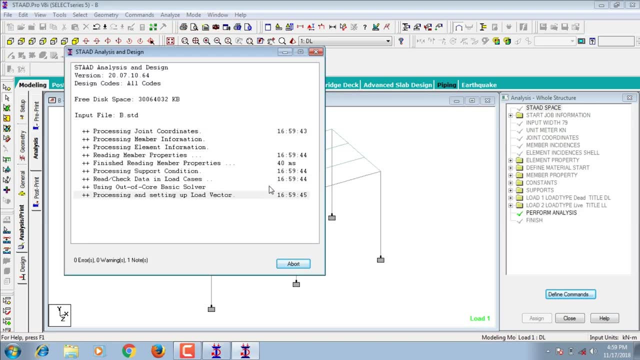 Assign: Yes, Ok. So after that go to analysis and print again. Just add it again, Close it again. Ok, Analyze again. Run analysis again, Save it. Please check for zero errors. for this model, Click on post processing mode. 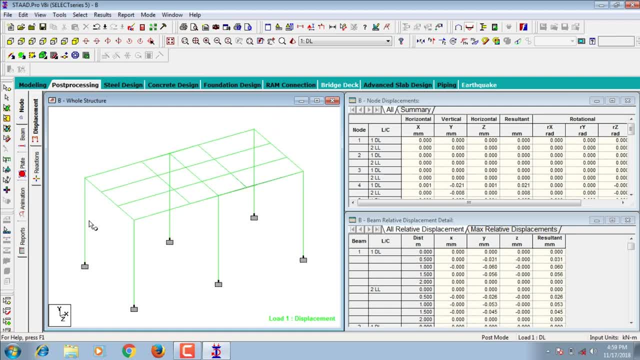 Done it Ok. Apply here. Click ok button. Ok, It indicates your deflection of the building. Ok, So I will show you the deflection. So this is the deflection of the building, Ok. So after that, click on F5.. 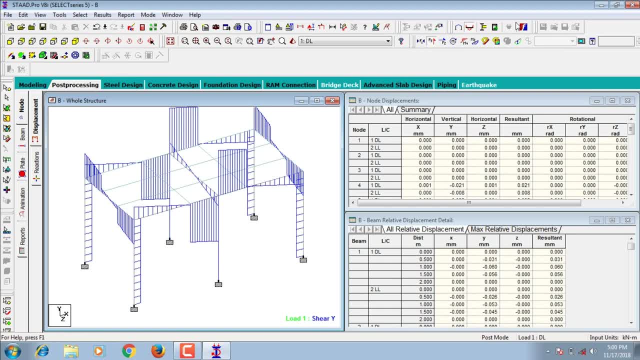 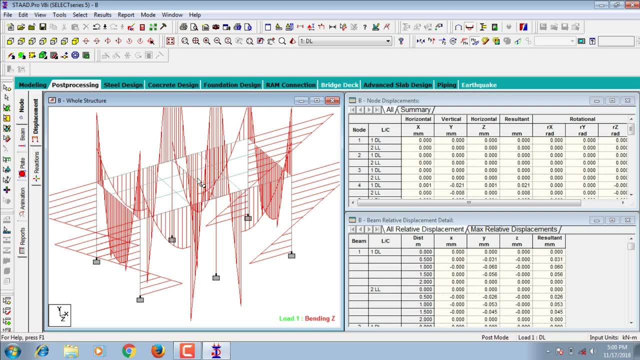 Ok, This is the shear force diagram for my building. Ok, Click on MZ value. Ok, This is the bending moment diagram for my building. Ok. So after that, click on nodes: Ok. Reactions: These are the support reactions for different joints. 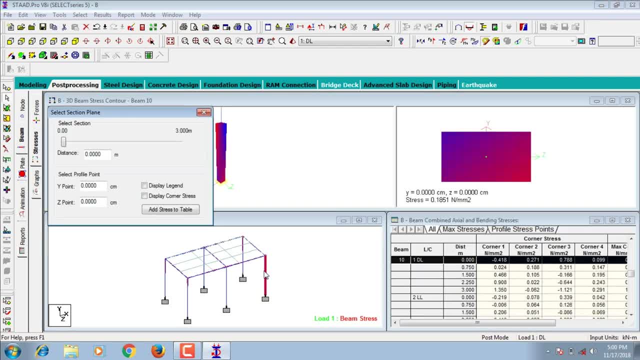 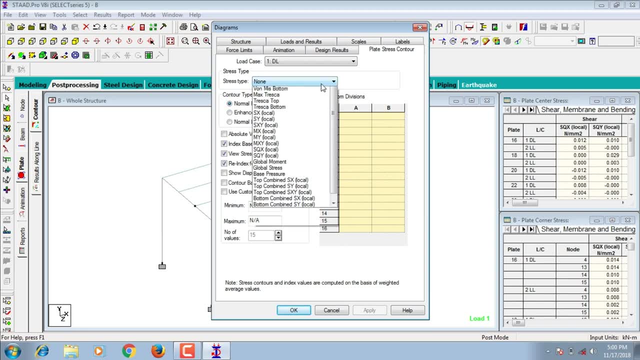 Ok. After that, click on beams. Ok, These are the stress diagrams for the beam, As well as columns: Ok. So these are the stress diagrams. After that, go to plate Select plate: Ok, So apply maximum absolute pressure on the plate. 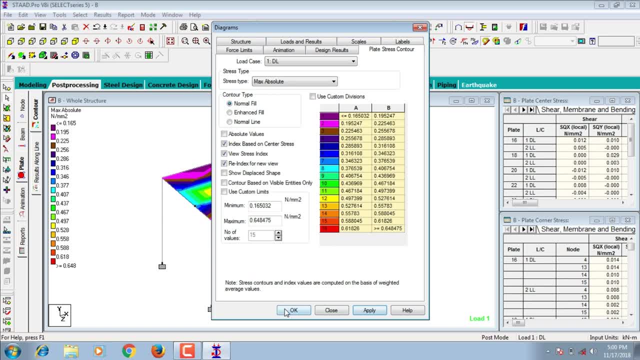 Ok, Just apply here. Ok, This is the maximum absolute pressure on the plate. Ok, So after that, go to modeling again, Go to design again, Go to select concrete. So in that we need to select IS 456-2000 code. 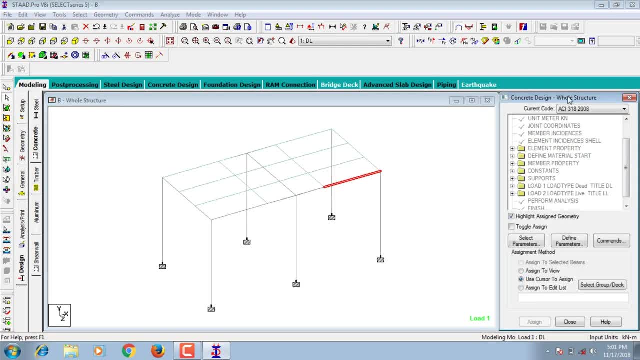 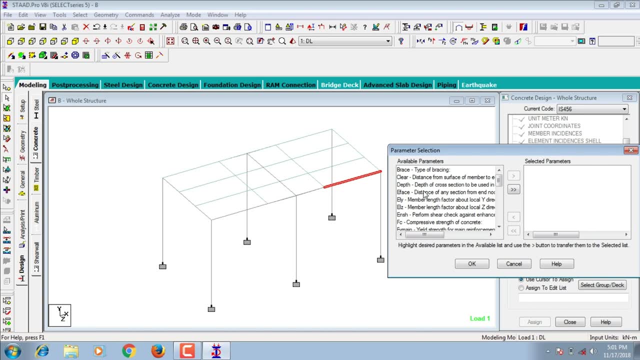 Click on select parameters. Initially we need to select all the parameters, So in this I am selecting clear. Ok, So I have selected clear. Ok, So I have selected clear. Ok, So I have selected clear. 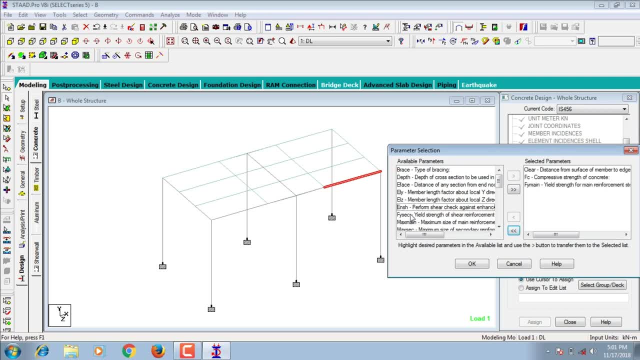 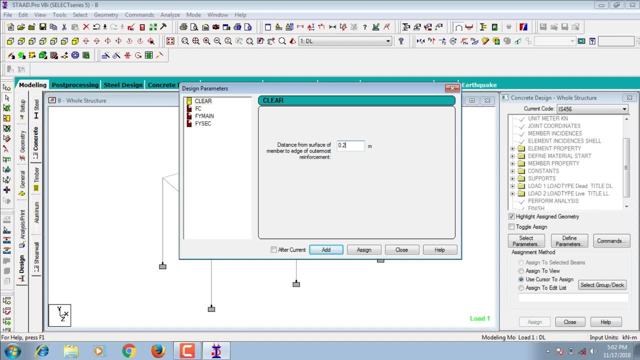 So I have selected clear. Okay, so compress the strength. yield strength: yield strength of shear reinforcement. Click OK button. After that go to different parameters. Just I am assuming 0.025.. Nothing but 25 mm is my cover. Just click on add button. Go FCK. So I am assuming M30 grade concrete. Okay, Just add it. Just I am assuming again 500 grade steel. Okay, So 500. Just add it. 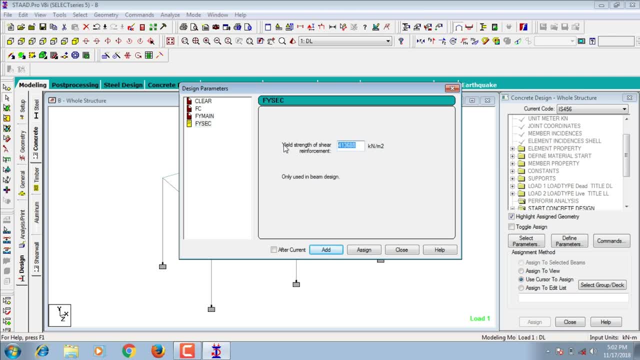 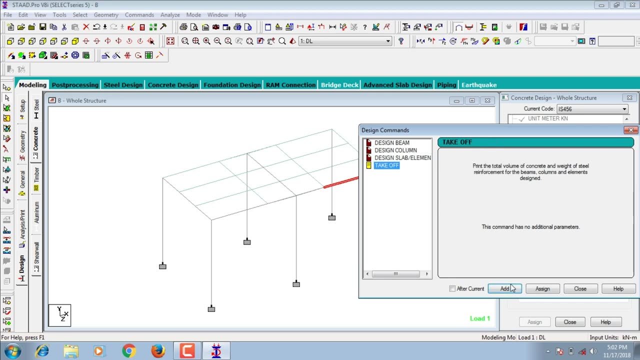 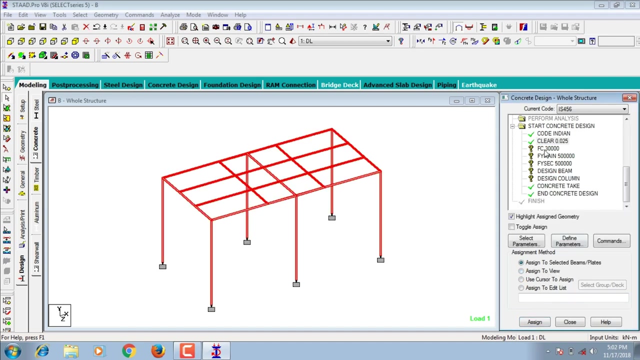 Okay, Shear reinforcement is also 1500 grade, Okay, Just add it Okay. Okay, Close it Okay. After that, click on commands: Okay, Add beam command. Again, add column command. Take off, Add it, Okay. So after that, select clear cover. Click on assign to view Assign. yes, Okay, Select FCK Assign to view Assign: yes, Okay, So FCK. 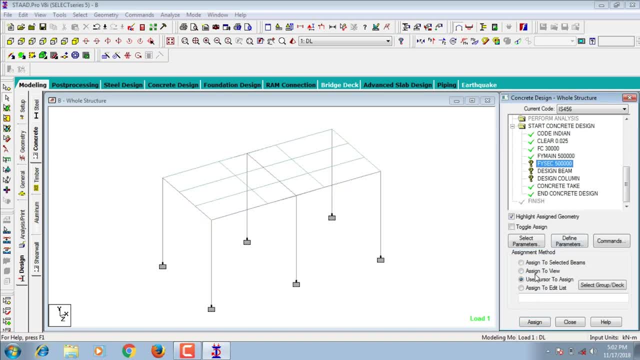 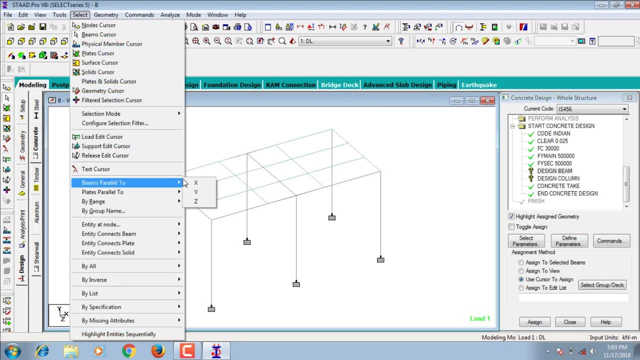 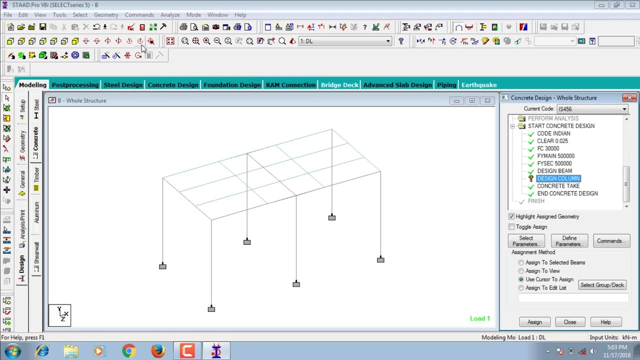 Main reinforcement Assign to view Assign: yes, Okay. So select F5 section: reinforcement Assign to view Assign: yes. Select beam command: Go to select option. Select beams parallel to X direction: Again. go to select beams parallel to Z direction. Assign to select beams Assign: yes, Okay. Select column command: Again. go to select beams parallel to Y direction Assign to select beams Assign: yes, Okay. So after this, go to design again, Again, concrete design: Okay, So select BS8007.. 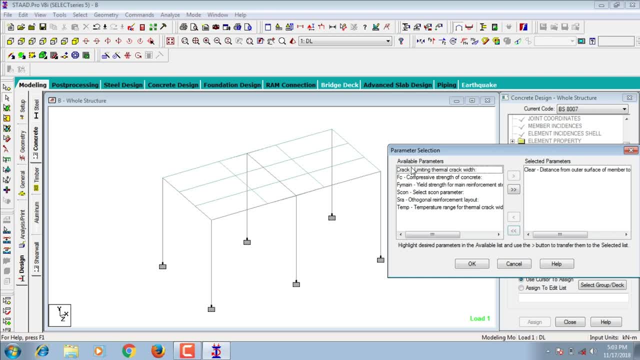 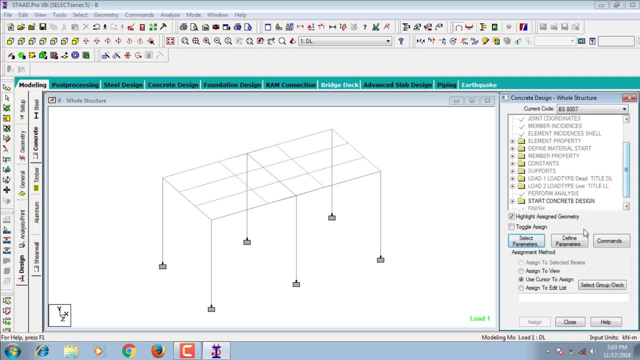 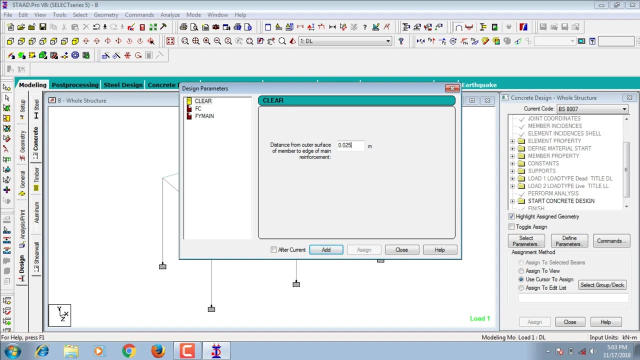 Okay, In that, select parameters, Okay. And you have to select clear distance, Okay, Compressor strength as well as yield strength of shear reinforcement. Click on okay button, Okay, So you can define parameters. Just, I am assuming again 25 mm. is the cover? 0.025. Just add it, Okay. Select the compressor strength. So here also I am assuming 30000.. M30 grade: Okay, So main reinforcement is 500 grade steel, Right. 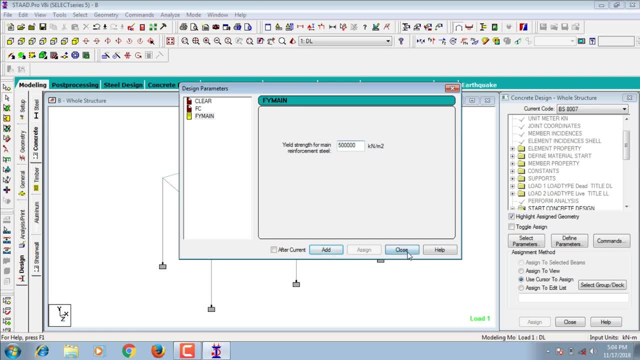 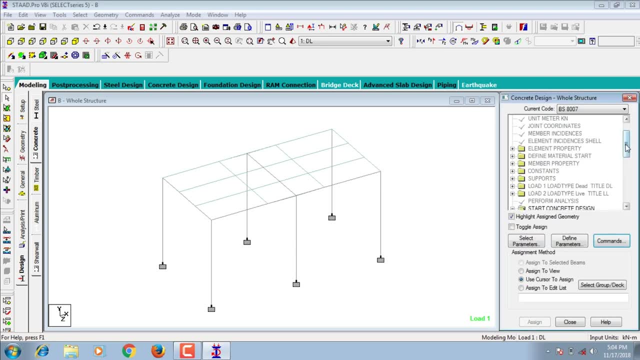 500.. Add: Okay, Close it Okay. So after that, click on commands. Okay, Select a slab command. Okay, Again, take off command, Just close it. Okay. So I will assign this all sections to My slab. Okay, Click on assign to view. 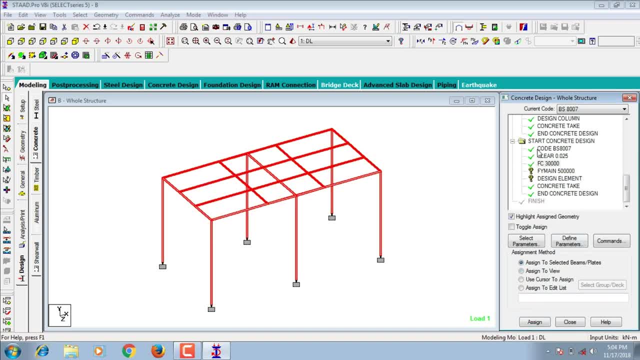 Assign: Okay Again. select compressors: strength: Assign to view Assign: Okay. Steel: Okay. Assign to view Assign: yes, Okay. So design element: assign to view assign: yes, okay. after that again click on analysis and print again analyzing. 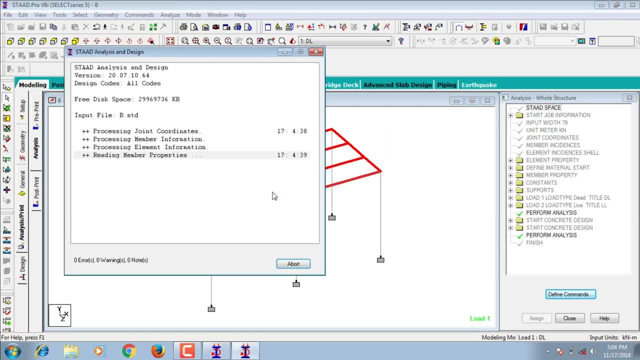 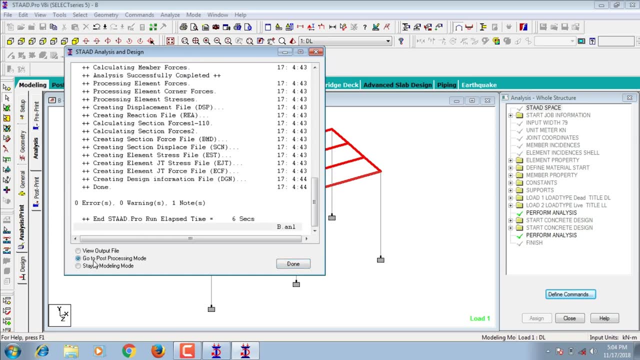 and close it again. so click on analyze, run analysis, save it. please check for zero errors again. if you are done with zero errors, then your module is correct. for design also: okay. click on go to post processing. one click on done button. okay. so after this we need to. 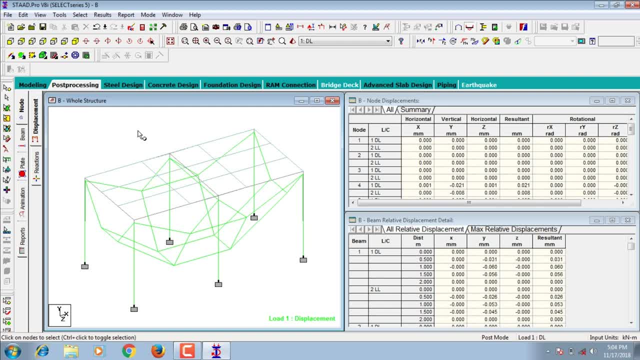 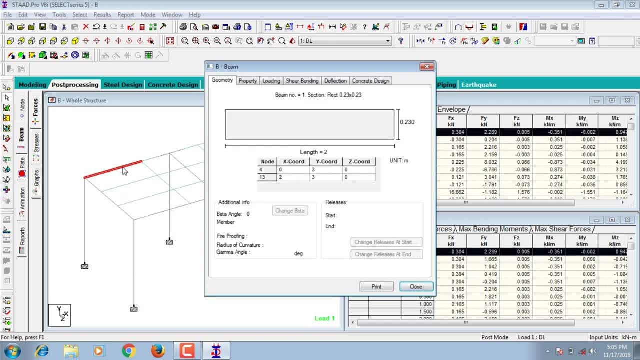 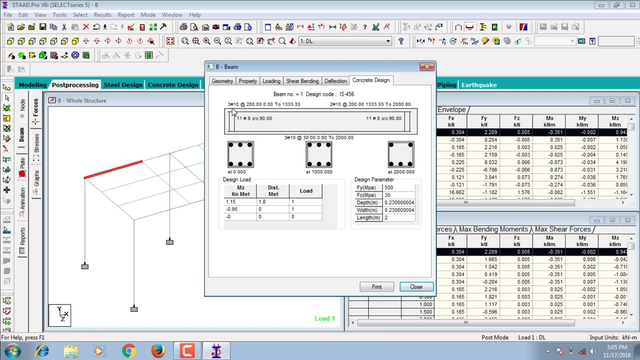 see the results which are related to beam design, column design, snap design: right, so for that, go to select beam. okay, select any one of the beam. for example, i am selecting, uh, one beam. okay, just double click on it. okay, these results indicates your beam design results. so it will be consisting of top reinforcement will be consisting of three bars of 10 mm. 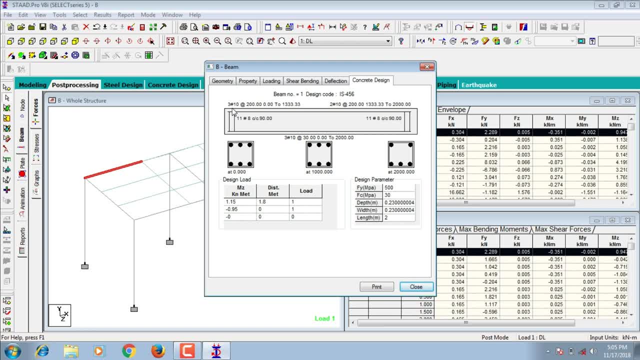 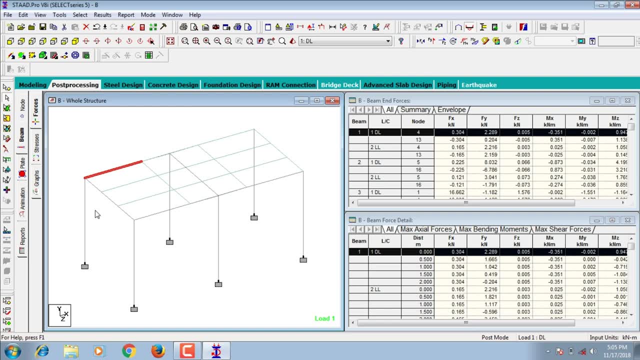 dia bottom reinforcement should be consisting of three bars of- okay, 10 dia bars. okay, so it will be consisting of six bars in each section. okay, close it. okay, after that, select any one of the column, just double click on it. click on concrete design. okay, so now you. 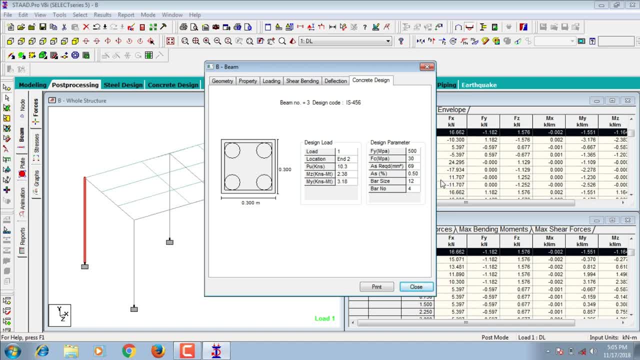 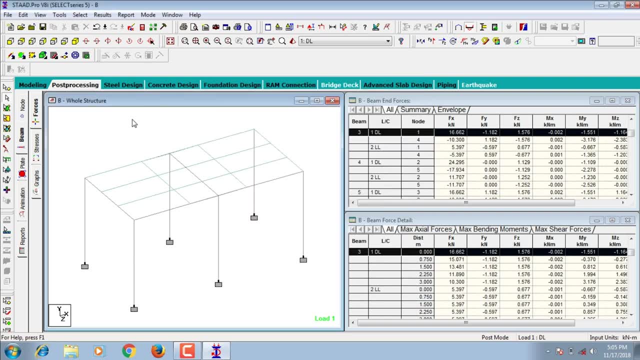 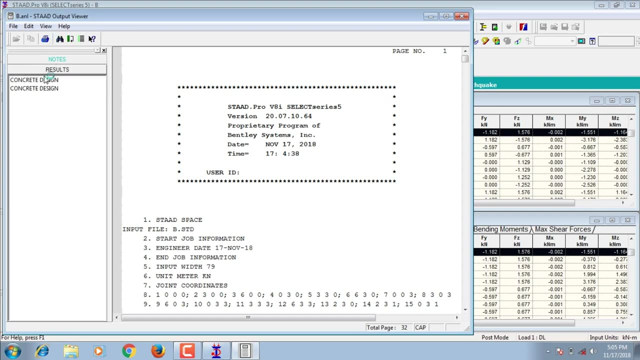 know the result. okay, so it will be consisting of девal. okay, so it will be consisting of column. will be consisting of four bars of 12 mm dia. okay, click on close bottom. so after that we need to see the results, which are related to beam and column as well as uh, slap. 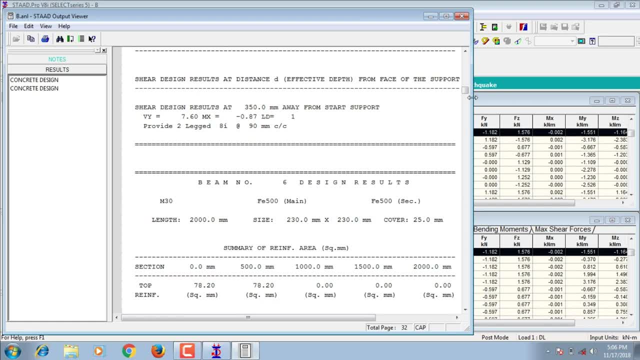 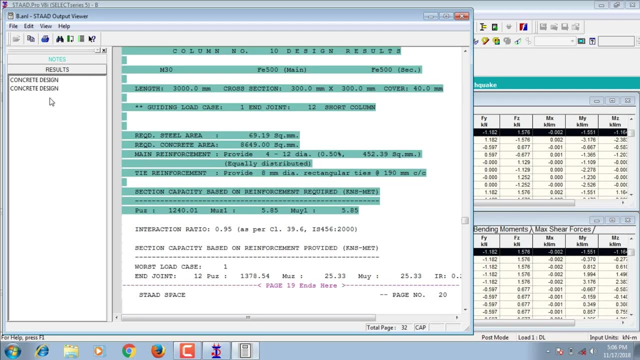 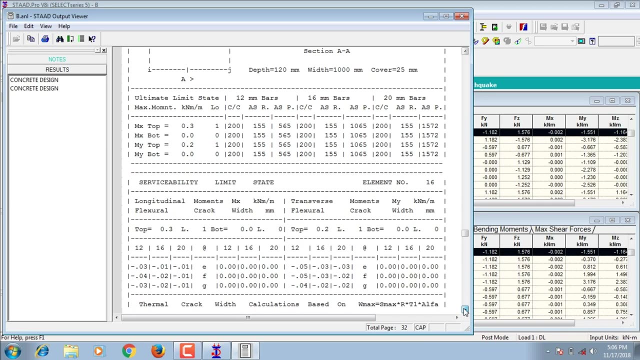 okay, further, go to start output file. okay, click on results. so click on first concrete design. so these results beam one indicates your beam design results. okay, as well as your results. okay. after that, again click on concrete design. again second concrete design. so these results indicates your slab design. okay, these are all our.